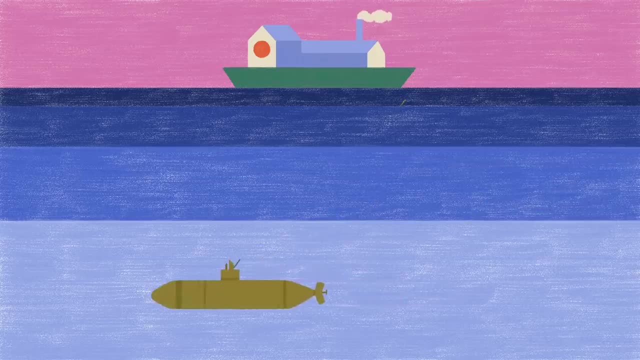 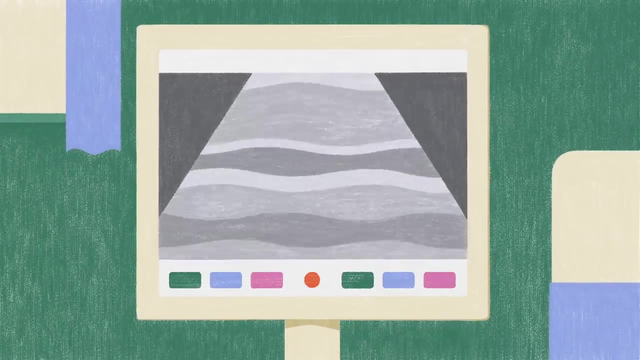 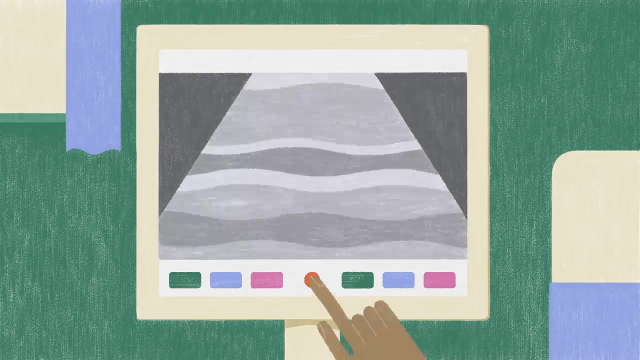 even faster through mediums with more tightly packed molecules like water. In the 1950s, medical professionals began to experiment with this technique as a non-invasive way to see inside a patient's body. Today, ultrasound imaging is used to evaluate organ. 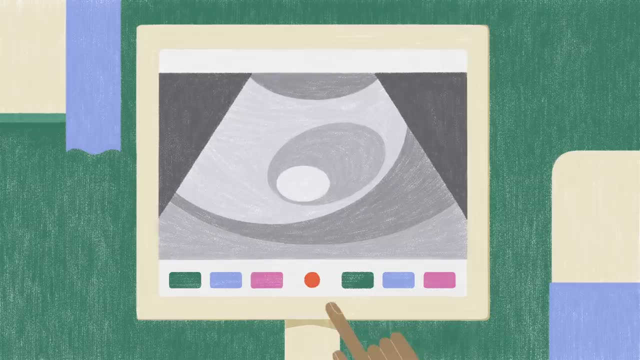 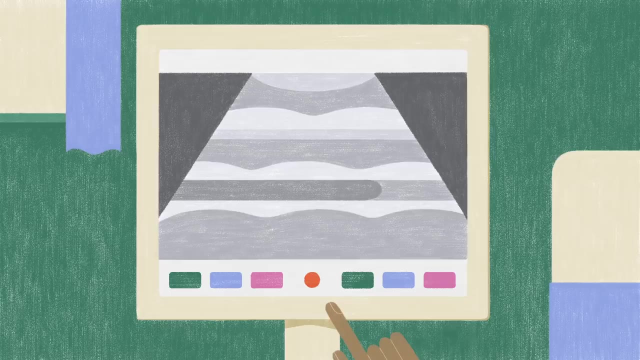 damage, measure tissue thickness and detect gall-bladder stones, tumors and blood clots. We've learned that ultrasound may be a more advanced technology than even an original, But to explore how this tool works in practice, let's consider its most well-known use — the fetal ultrasound. 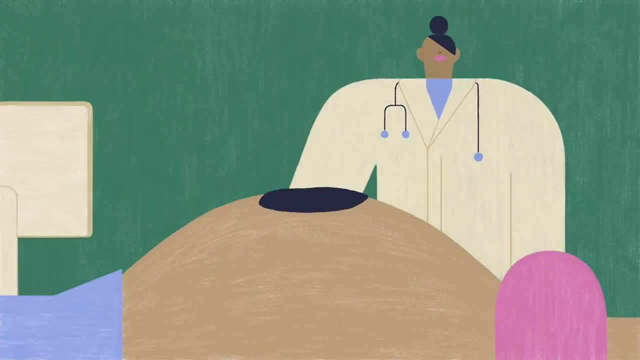 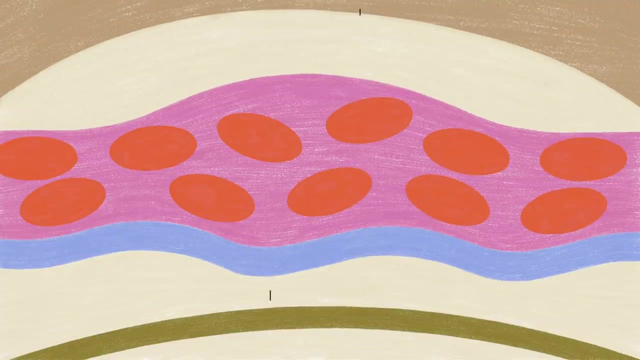 First, the skin is covered with conductive gel. Since sound waves lose speed and clarity when traveling through air, this gooey substance ensures an airtight seal between the body and the wand emitting ultrasound waves. Then the machine operator begins sending ultrasound beams into the body. 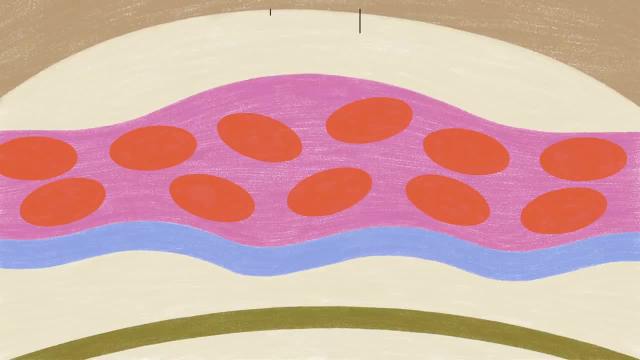 The waves pass through liquids like urine, blood and amniotic fluid without creating any echoes, But when a wave encounters a solid structure, it bounces back. This echo is rendered as a dot on the imaging screen. Objects like bones reflect the most waves. 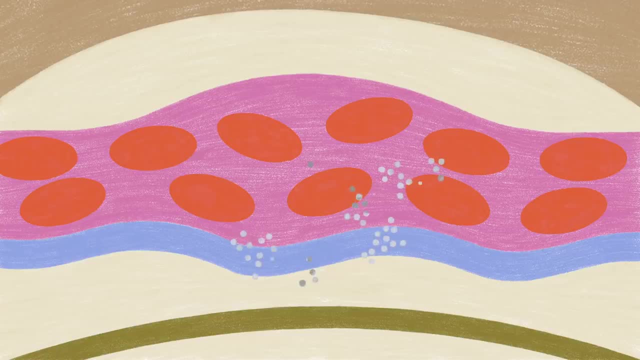 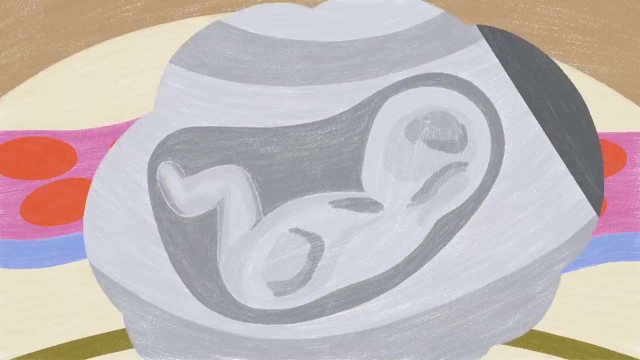 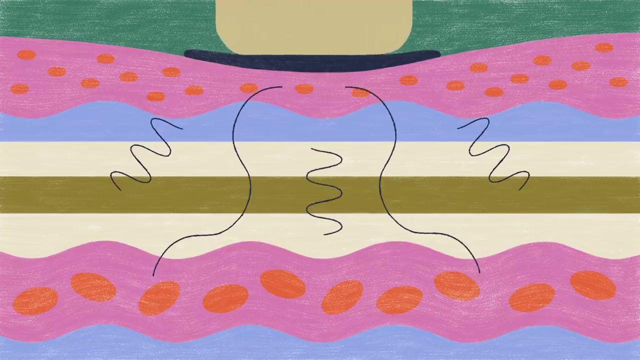 appearing as tightly packed dots forming bright white shapes. Less dense objects appear in fainter shades of gray, slowly creating an image of the fetus's internal organs. To get a complete picture, waves need to reach different depths in the patient's body, bypassing some tissues while echoing off others. 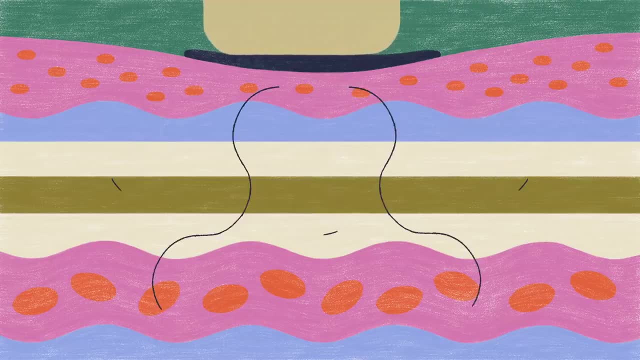 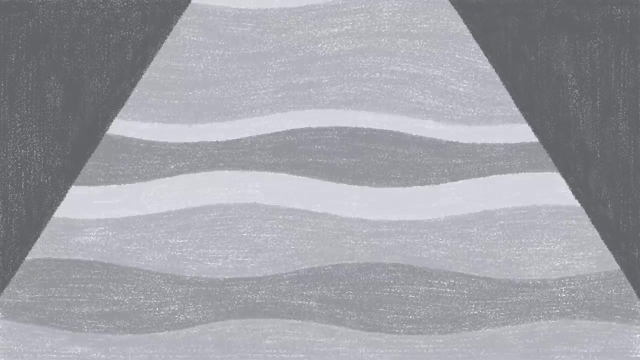 Since longer low-frequency waves actually penetrate deeper than short high-frequency ones, multiple frequencies are often used together and composited into a lifelike image. The operator can then zoom in and focus on different areas. And since ultrasound machines send and receive waves, 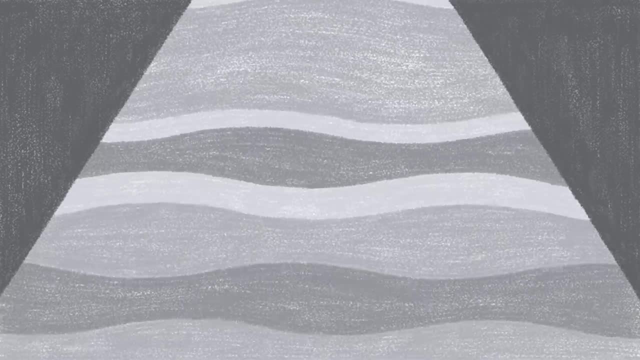 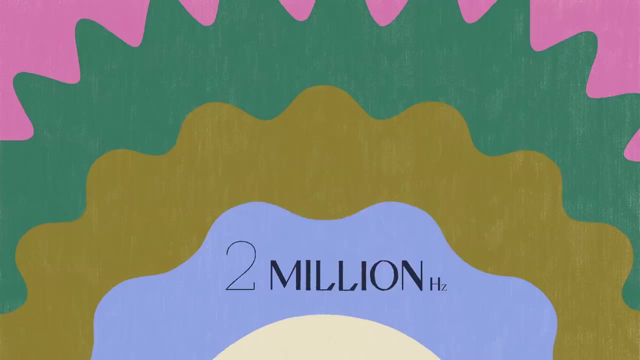 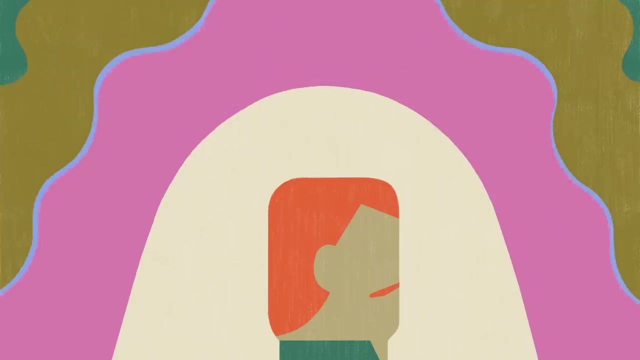 with cascades of waves in real-time. the machine can even visualize movement. The waves used for medical ultrasound range from 2 million to 10 million hertz- over a hundred times higher than human ears can hear. These incredibly high frequencies create detailed images that allow doctors to diagnose.